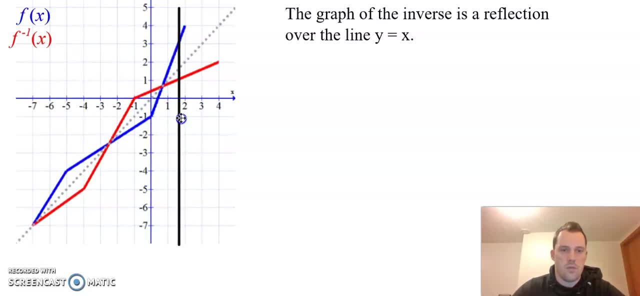 point, does our vertical line touch the blue graph more than once? Similarly, when we have our inverse graphed, we know for sure this is an inverse, because it also passes the vertical line test. Well, there's a way to test if a function has an inverse without having to actually graph it. 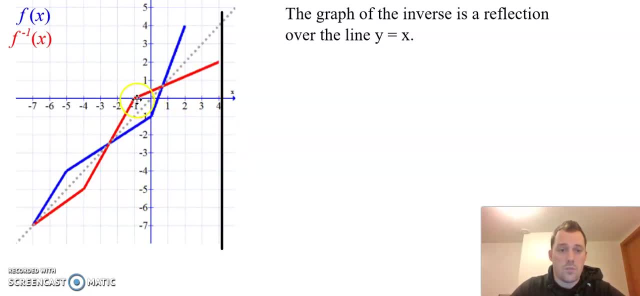 So recall that these points, the x and y values are just flipped around. You can think about it like a graph. So you can see that the x and y values are just flipped around. So you can think about it like a graph. So you can think about it like a graph. So you can think about it like a graph. 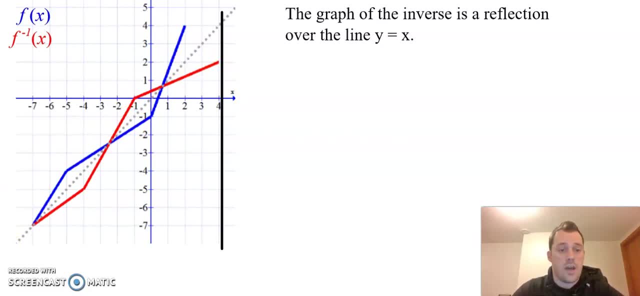 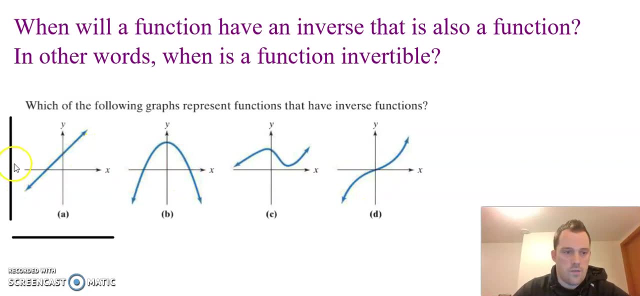 So that's how we're able to use the horizontal line test to check if we have an inverse. So let's just double check that all of these are indeed functions. So we have our vertical line. at no point does the vertical line touch any of these graphs at more than one. 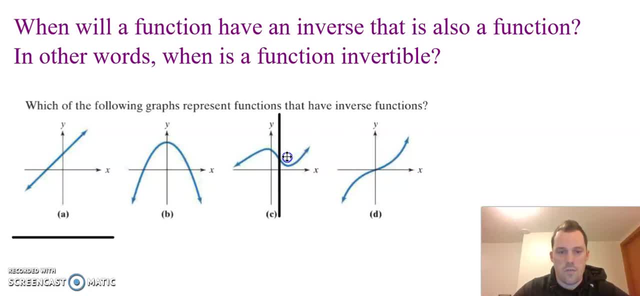 point at the same time. That tells us all these are functions. But now if we take horizontal line- and that passes as well- where we don't touch our graph more than once at any point, then we do in fact have an inverse. So this has an inverse here, This parabola. 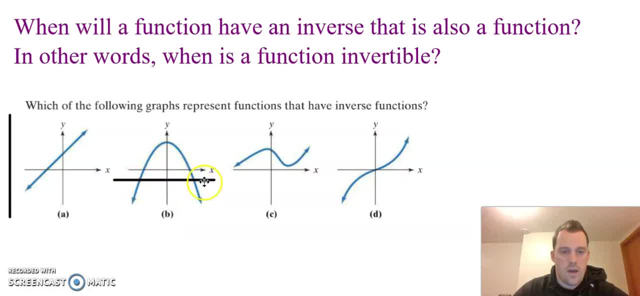 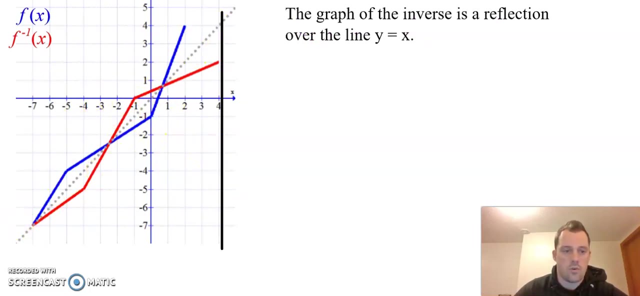 we notice that our horizontal line touches the graph at two points, pretty much the entire graph. So that tells us that even though we could just take this y equals x line and reflect across or take key points of this graph, switch the x and y around and actually graph it out, 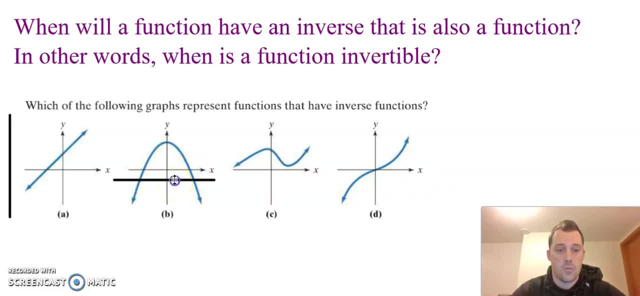 That doesn't mean that it is an inverse of this function. So because this does not pass the horizontal line test, there is no inverse for this parabola. Similarly, with this one we're touching at two or three points, pretty much the entire graph. 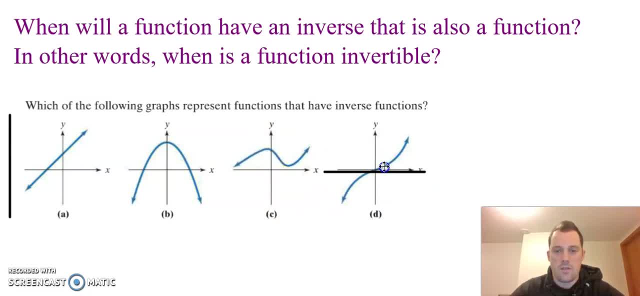 So this does not have an inverse and this graph does have an inverse.